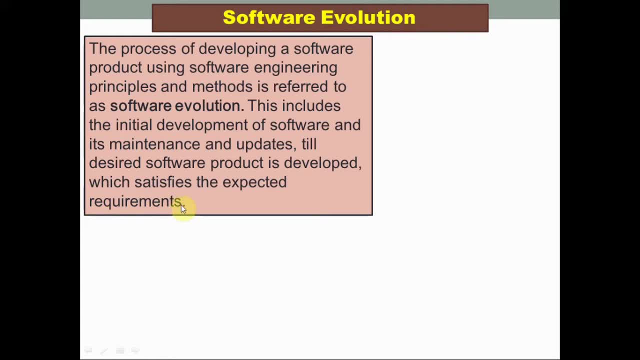 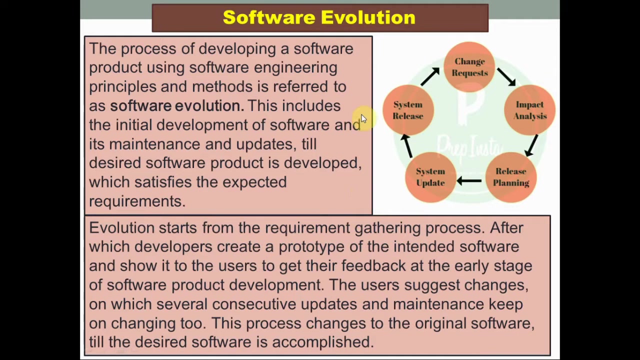 In software evolution, software's initial development, maintenance and updates are included until desired software product is developed. Also, such software product has to be developed which satisfies the desired user's requirements. You can see in this picture how software evolution takes place. 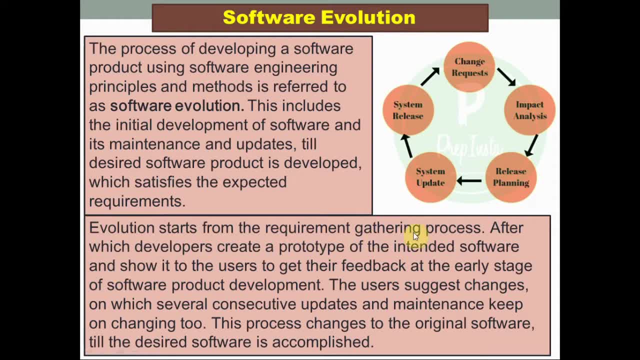 Evolution starts from the requirement gathering process, After which developers create a protocol to develop the model, create a prototype of the intended software and show it to the users to get their feedback. at the early stage of software product development, The users suggest changes, on which several consecutive updates and maintenance keep on. 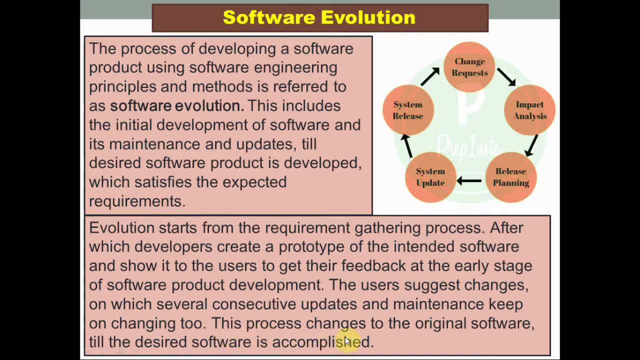 changing too. This process changes to the original software till the desired software is accomplished. Software evolution starts with the requirement gathering process. After that, developers create a prototype of the intended software and show that prototype to the users. Users give feedback on that prototype. 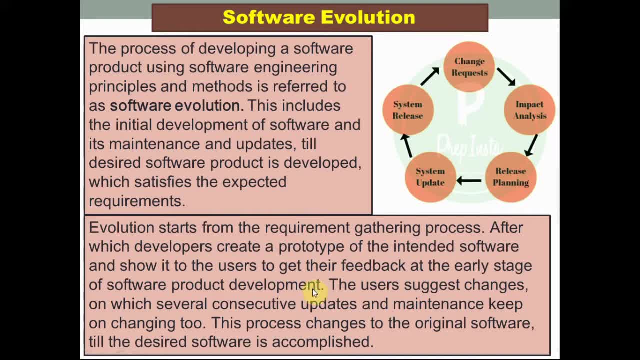 This process takes place at the very early stage of the software development process. Users then suggest changes to the prototype If changes are to be made. they also suggest changes. According to the feedback of the users, consecutive updates and changes are made to the software. 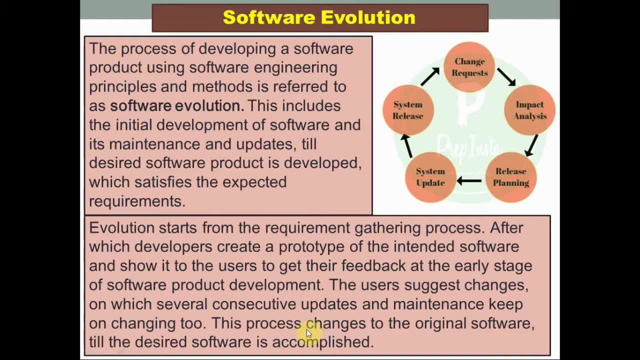 These changes keep on happening till the desired software is completed. This process takes care of the sua performance of the software product. The pace of software evolution will help to develop the desired software the way it should be developed: Audio, Infotainment- The names of software evolution. 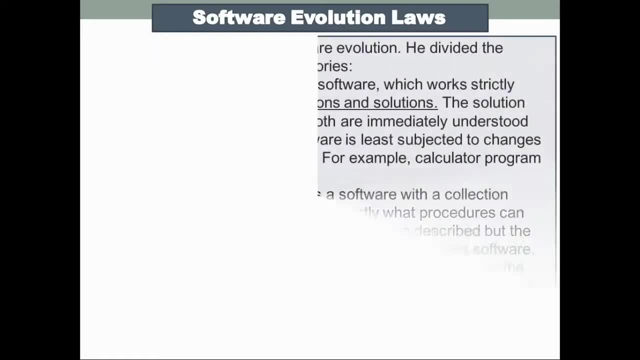 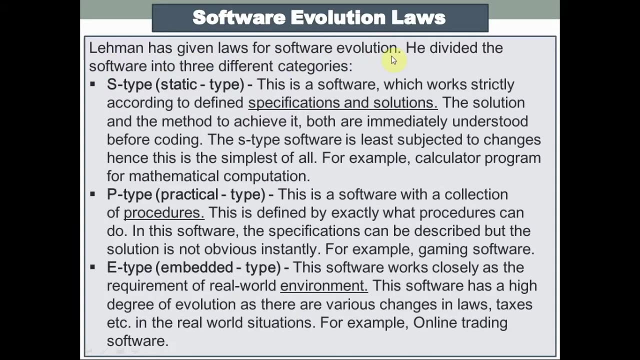 give rise to United System account headphones. The chart users are displayed color. Legends, Theots hear, are the results of that software evolution. Lemon has given laws for software evolution. He divided the software into three different categories. Lemon formulated some software evolution laws in 1974.. 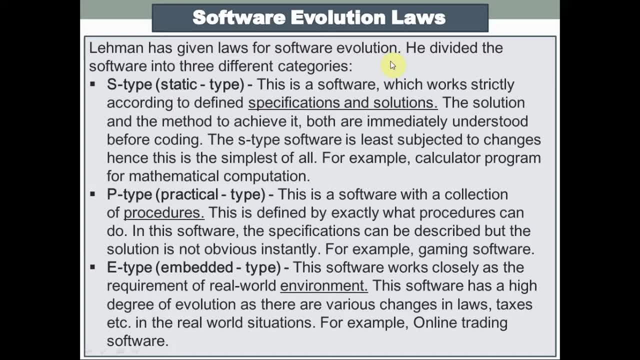 And in his 1980 article, Lemon qualified the application of such laws by distinguishing between the categories of software or software ki wo categories: thi S-type, P-type and E-type. S-type category is the short form of static type software. This is a software which works strictly according to defined specifications and solutions. 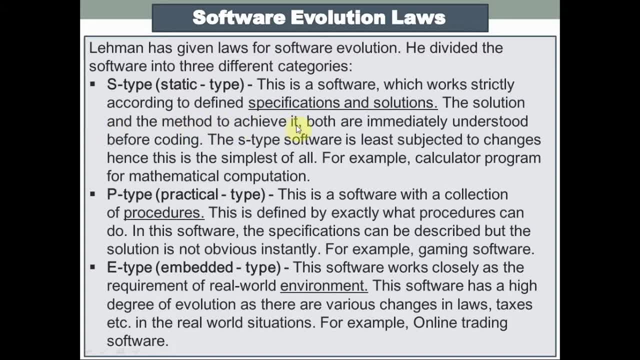 The solution and the method to achieve it. Both are immediately understood before coding. The S-type software is least subjected to changes, Hence this is the simplest of all. For example, calculator program for mathematical computation. S-type software works according to defined specifications and solutions. 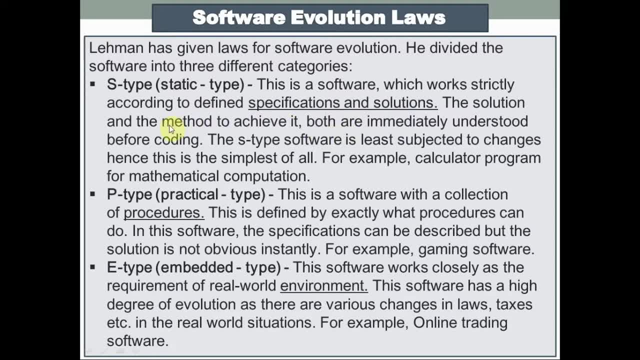 It is most톱h the simplest of all. It is similar to the P-type software, S-type software, except the type of software used. inaluzation is not possible. However, S-type software is the most complex. makes somythed clicked. 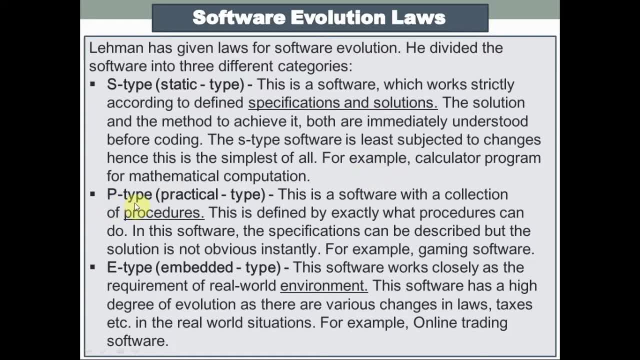 It is competitive software. It is their power of fart. People are two, as if tighmmot. the decay Ptype is the shortest form of practical type software. This is a software with a collection of procedures. This is defined by exactly what procedures can do. 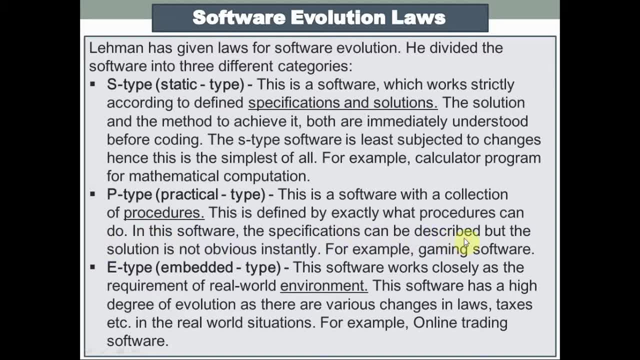 In this software the specifications can be described, but the solution is not obviously instantly. For example, gaming software, Practical type software, has a collection of procedures and it defines what the procedures do. In ptype software, the specifications can be described, but the solution is not obviously. 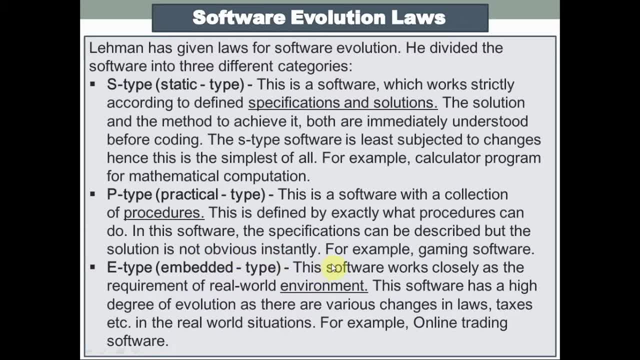 instantly. In ptype software the specifications can be described, but the solution is not obviously instantly. In ptype software the specifications can be described, but the solution is not obviously instantly. Ptype software doesifiye for maintenance of physical assets. In ptype software the specifications can be described, but the solution is not easily. 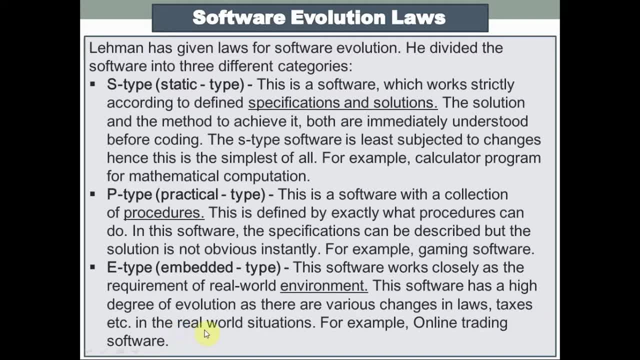 instantly, etc. in the real world situations. for example, online trading software, embedded type of software which works on the real world environment, and the evolution of this software is high degree of evolution because it can handle the changes of the real world in a good way, and example is online trading software. so you can see in online trading software 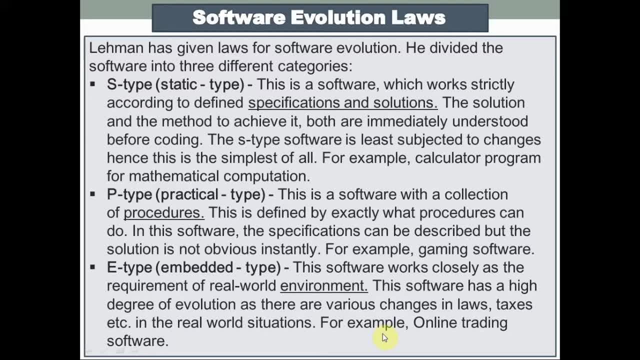 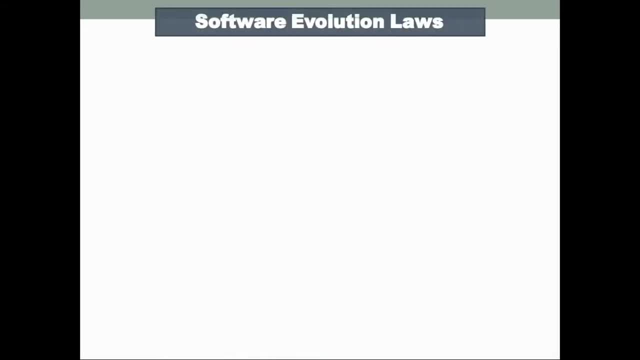 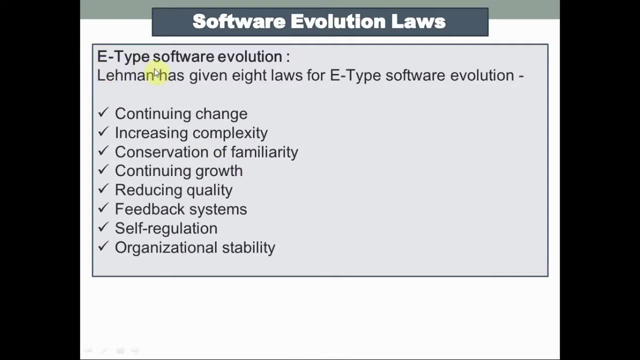 how it works on the requirements of real world e type software evolution. Lemmon has given 8 laws for E-Type Software Evolution. So Lemon gave 8 laws and those laws only work on E-Type Software. The laws are Continuing Change, Increasing Complexity, Conservation of Familiarity.